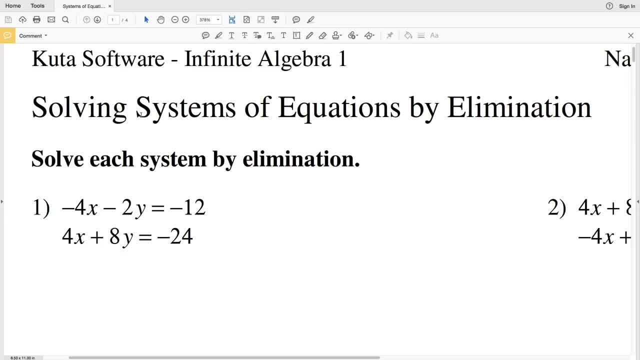 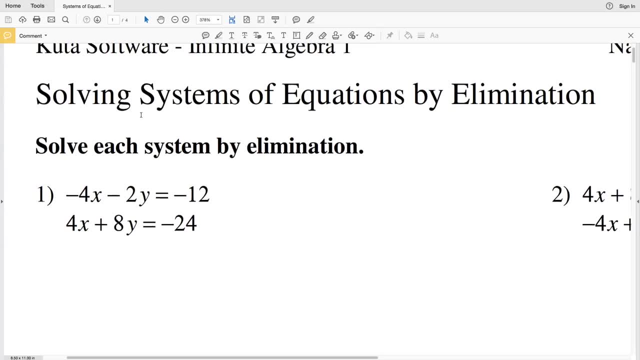 In this video we're going to start the CUDA software Infinite Algebra 1 free worksheet solving systems of equations by elimination. Our directions for this video are to solve each system by elimination and I'll leave a link in the description below so you know how to access. 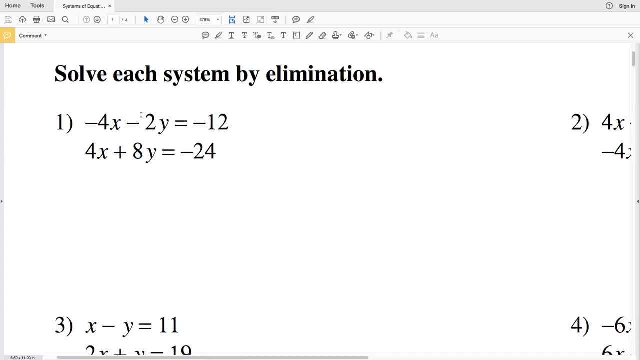 this worksheet, If we're solving by elimination, essentially we're going to be canceling out a variable so that we have the equation only in terms of one variable. So in number one we have negative. 4x minus 2y equals negative 12 and 4x plus 8y equals negative 24.. However, if you 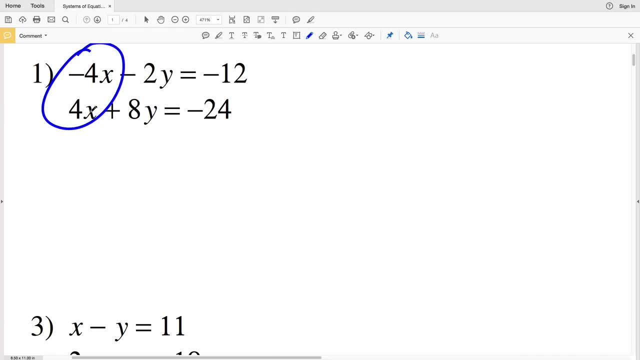 know, if I add these two equations together, negative 4x plus 4x equals 0 and 0x is simply 0. and then if I'm taking away 2y, so negative 2y plus 8y will be 6y and that's going to be equal. 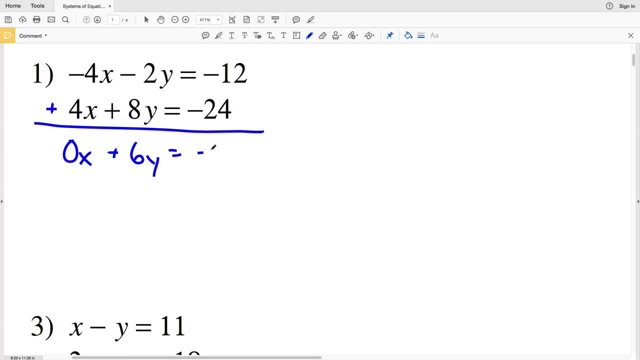 to negative 12 plus a negative 24. Which is a negative 36.. 0 times x is 0, so I have that 6y is equal to negative 36.. So what I'll do is I'll divide by 6 on both sides so that I can solve for y and get that y is equal to negative. 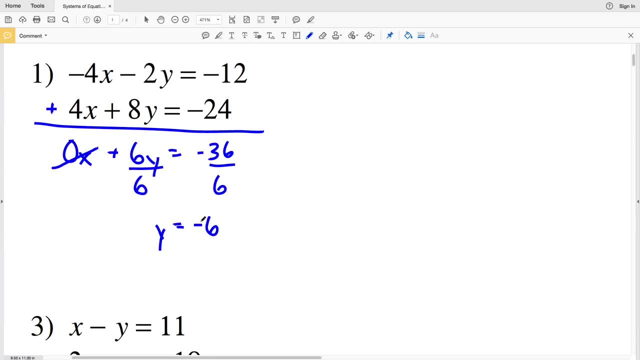 6. Since negative 36 divided by 6 is negative 6. Now that I have what y is, I can plug that back in to the top equation or the bottom equation and solve for x. Let's go ahead and plug it into this. 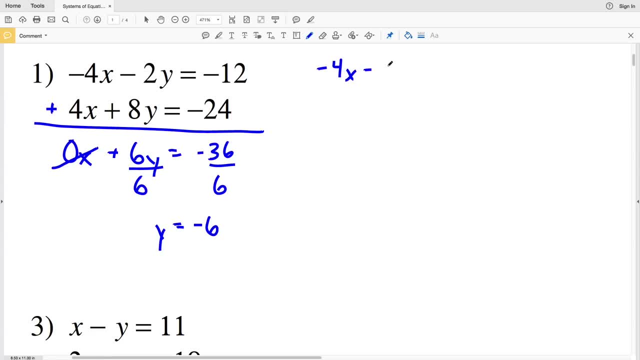 top equation. So I'll have negative 4x minus 2 times negative 6, since y is negative 6 and that's equal to negative 12.. So negative 4x minus 2 times negative 6 is negative 12, but if I'm subtracting a negative 12, 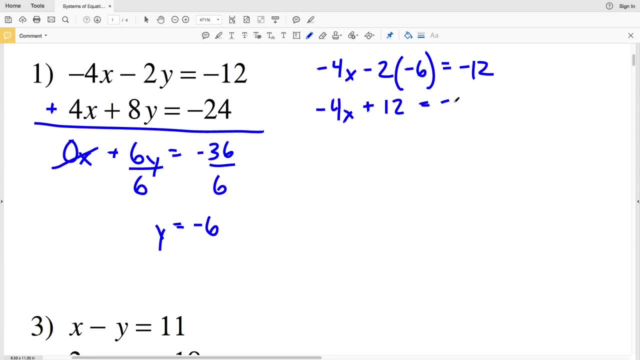 it's the same as adding a positive 12 and that's equal to negative 12.. So I need to isolate my term with the x, so I'll subtract 12 from both sides, So I'll get that negative 4x is equal to negative. 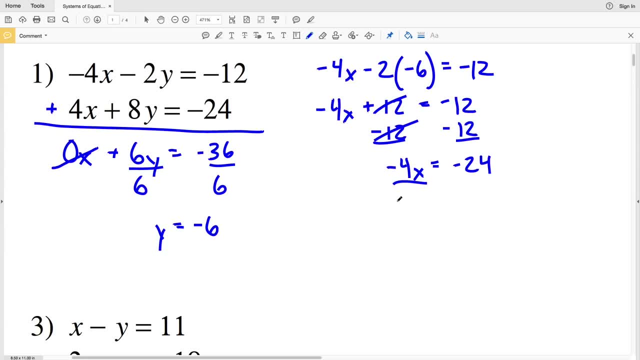 24.. Negative 12 minus 12 is negative 24.. And when I divide by negative 4, I'll get that x is equal to negative 24 divided by negative 4, which is a positive 6. So I have that x is equal to 6 and y. 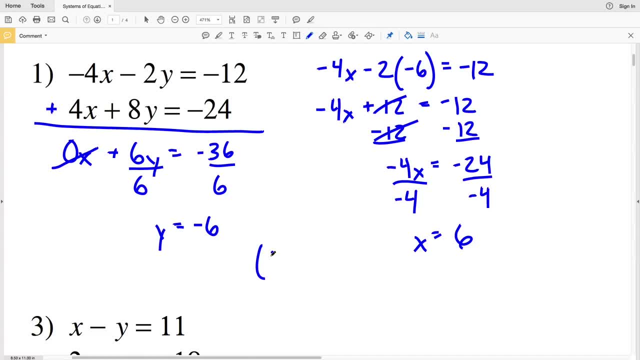 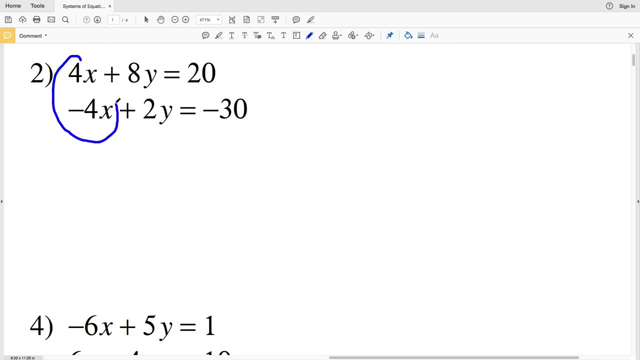 is equal to negative 6.. So, writing this as one answer, I'll just say 6 for x, comma negative 6 for y. x equals 6 and y equals negative 6 in number 1.. Again we can see that 4x plus negative 4x will equal 0. So if I'm adding these two equations, 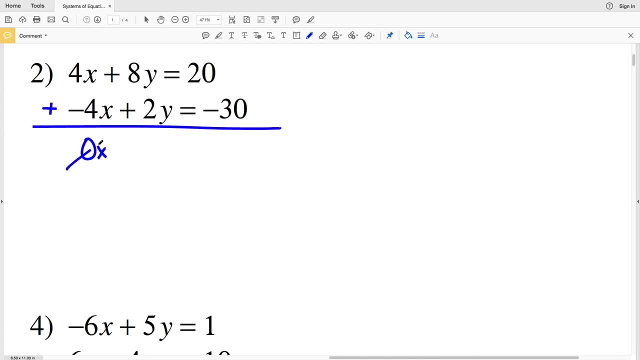 I'll get 0x, which we know is 0, and that will be added to 8y plus a positive 2y. So 10y is going to be equal to 20 plus a negative 30, or 20 minus 30, which is negative 10.. I'll divide both sides. 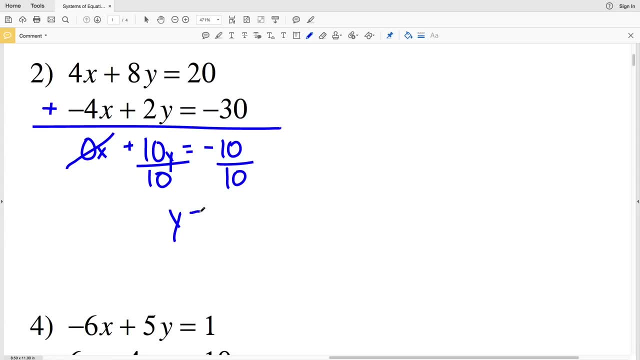 by 10 in order to isolate that y variable. So y is going to be equal to negative 10 divided by a positive 10.. Which is a negative 1.. Now that I have that y is equal to negative 1, I can plug y in to the top. 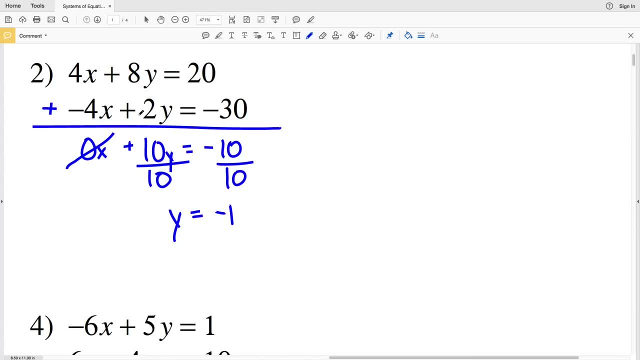 equation or to the bottom equation. Let's go ahead and just plug it into that second equation. So we'll have negative 4x and we're solving for x- so x's are unknown- plus 2 times negative 1, since y is negative 1 and that's equal to negative 30. So I'll have negative 4x plus 2 times negative 1. 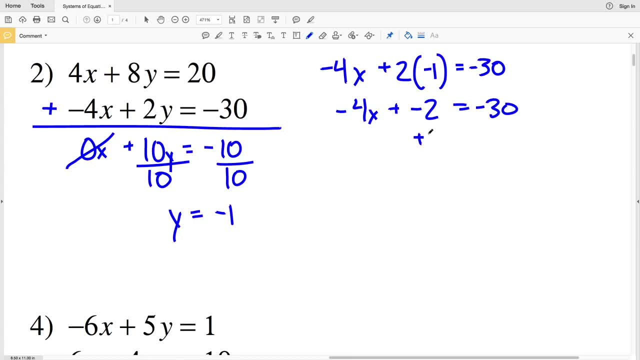 is negative 2 and that's equal to negative 30. So I'll add 2 to both sides and get that negative 4x is equal to negative 28.. And when I divide by negative 4, negative 28 divided by negative 4 will give me that x is equal to a positive 7.. So my 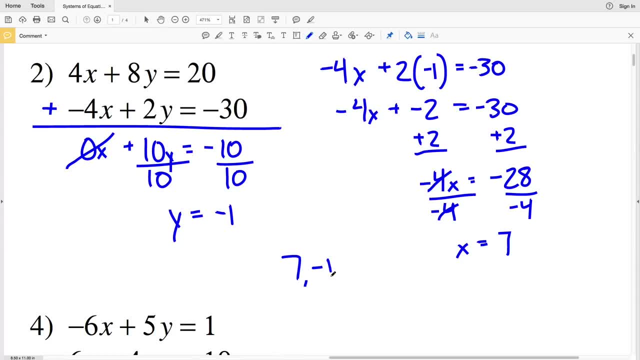 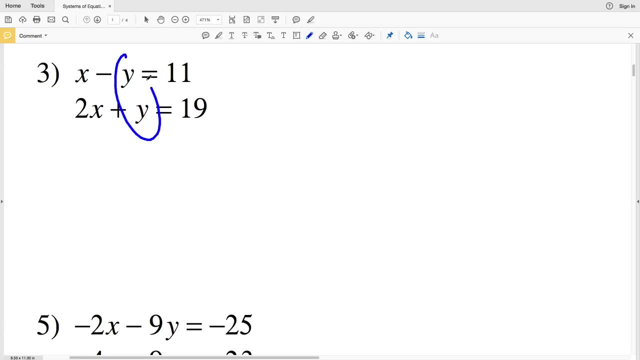 solution is 7 for x and negative, 1 for y And number 3. this time I'll be able to cancel out my y variable By adding the equations together: x plus 2x is 3x, negative, y plus y is 0 and 11 plus 19 is 30. So 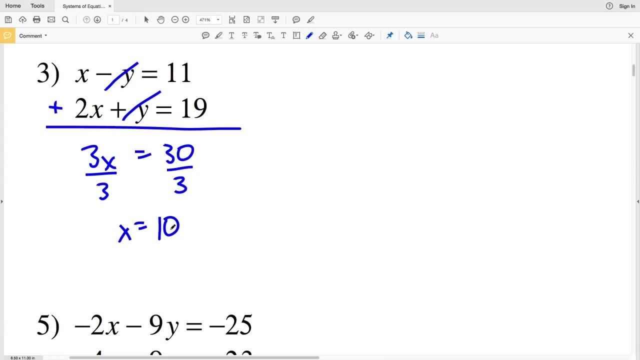 dividing by 3, I'll get that x is equal to 10.. Now I'm going to plug my value of x into either the first equation or the second equation, and plugging it into either equation will give me the same answer for y. So if we plug it into it- the top equation- we'll have 10 minus y, equal to 11, and 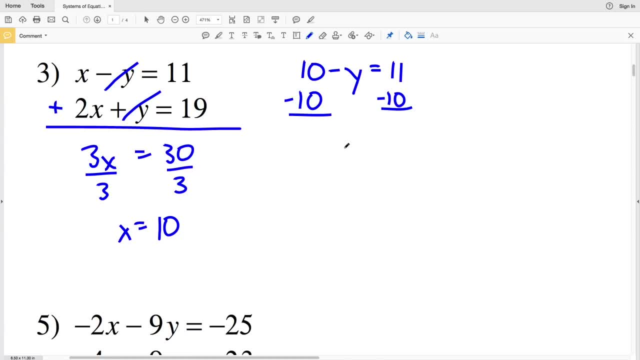 so I'll subtract 10 from both sides to get that negative y is equal to a positive 1.. Now I don't want my y to be negative, so I'll divide by a negative 1.. So I'll have that y is equal to a. 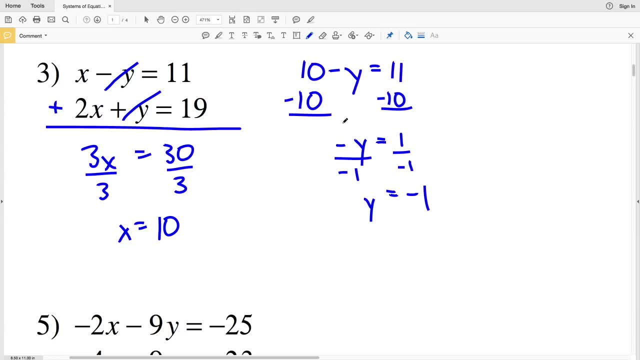 negative 1.. Or I could have also multiplied by a negative 1 and I still would have gotten that y is equal to negative 1.. So my solution number 3 is 10 for x and negative 1 for y. And, like I said, 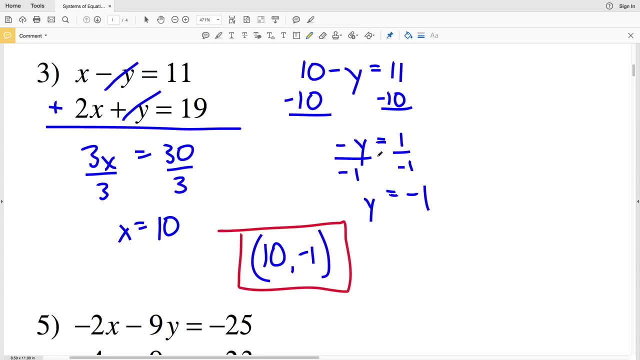 we also could have plugged x into this second equation and gotten the same answer for y. If x is 10, 2 times 10 is 20, and if we subtract 1 from 20, we will indeed get 19.. And number 4 I'll be. 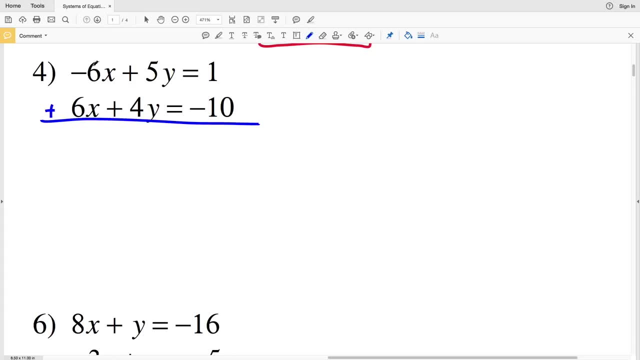 canceling out my x values by adding these two equations together: Negative 6x plus 6x is 0x or 10, which is negative 9. dividing both sides by 9, I'll get that Y is equal to negative 1, so I'll. 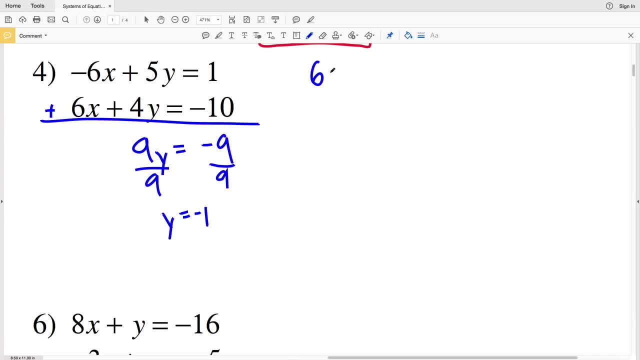 take that value and I'll plug that back in to the second equation. so I have 6x plus 4 times negative 1 equal to negative 10. that's 6x plus negative 4 equals negative 10. and when I add 4 to both sides, 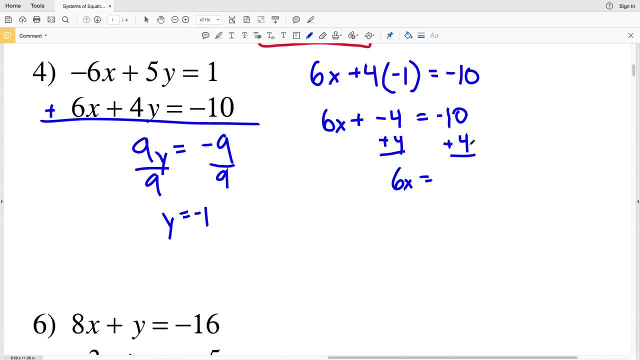 I'll get that 6x is equal to negative 6, so all I need to do is divide by 6 to isolate my X variable to get that X is equal to negative 1, so negative 1 is equal to X and negative 1 is equal to Y in. 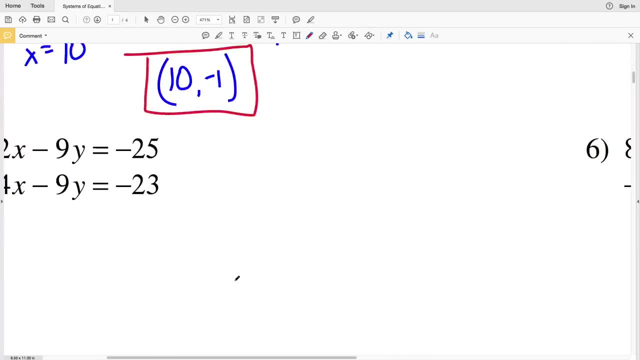 number 4, now in number 5, if I add these together my Y's will not cancel out. but if I subtract this equation they will cancel out. so I have negative 2x minus a negative 4x. so I can think of that is negative. 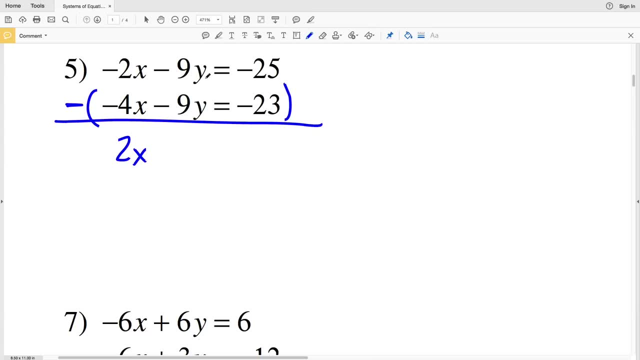 2x plus 4x, which will be a positive 2x. negative 9 Y minus negative 9y is going to be equal to 0. so plus 0 Y or minus 0 Y, and that's equal to negative 25 minus a negative 23, which is negative 25 plus. 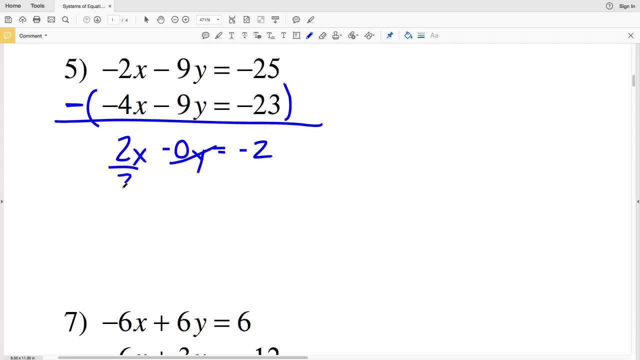 positive 23 is negative 2, so I'll divide both sides by 2 in order to isolate my X variable and get that X is equal to negative 1. since negative 2 divided by 2 is negative 1, now I'll take that value and plug. 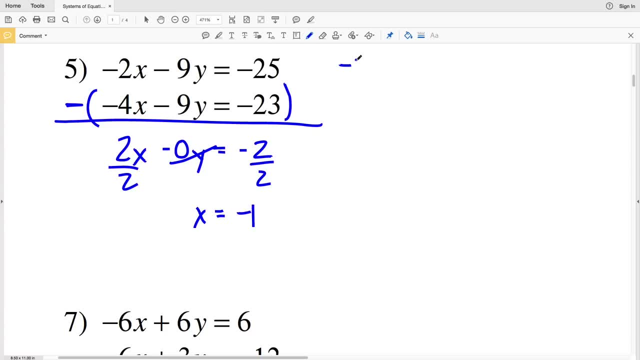 it back in. let's do the top equation. so: negative 2 times negative, 1 minus 9y equals negative 25. negative 2 times negative: 1 is a positive 2 and we're still subtracting 9y and that would be equal to negative 25. my next step will be to subtract 2 from both sides to get that negative. 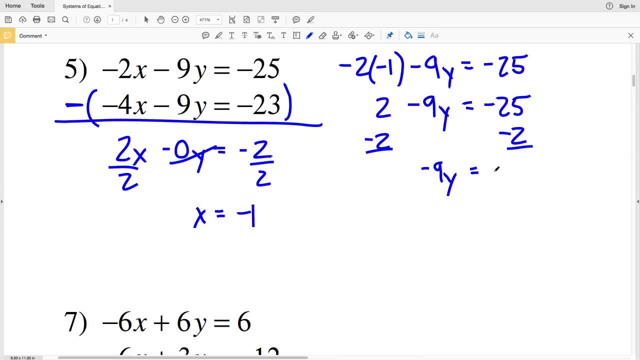 9y is equal to negative 25 minus 2, which is negative 27, and lastly, I'll divide by negative 9 in order to get my Y all by itself. and negative 27 divided by negative 9 is a positive 3, so my 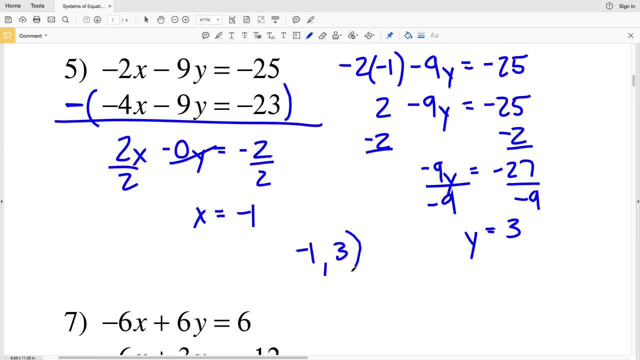 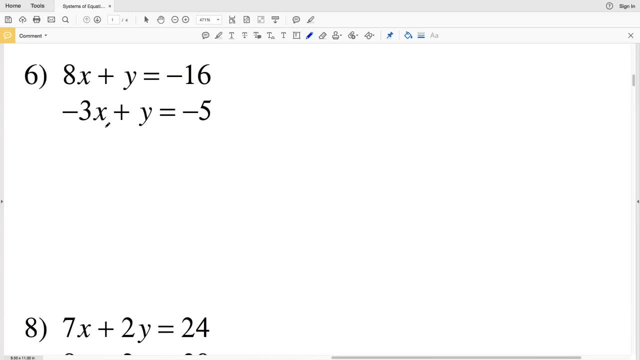 solution and number 5 is negative, 1, 3 negative, 1 is equal to X and 3 is equal to Y. and number 6 again, I'm going to be subtracting these equations. so if I have 8, X and I'm subtracting a, 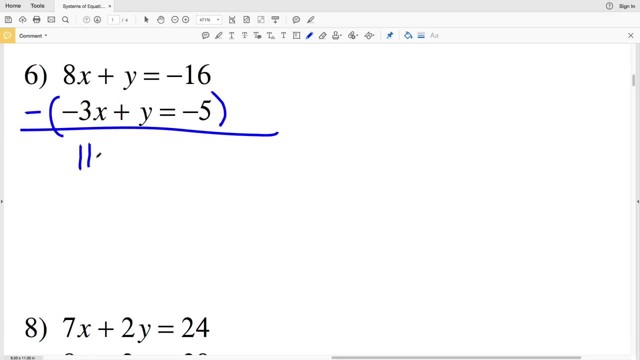 negative 3, that's 8 X, plus a positive 3, which is 11 X, and I have Y minus Y, which is 0, and that's going to be equal to negative 16 minus a negative 5, which is negative 16, plus a positive 5, which is. 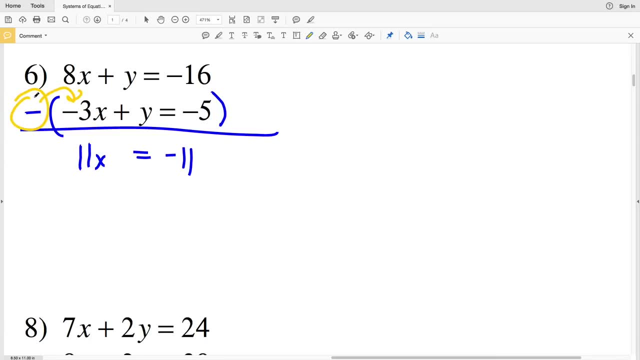 negative 11. you could also think of this subtraction as distributing a negative and then add each of the terms. either way, you will get 11, X equal to negative 11. then when I divide by 11, I'll get that X is equal to negative 1. so I'll take that value of negative 1 and plug. 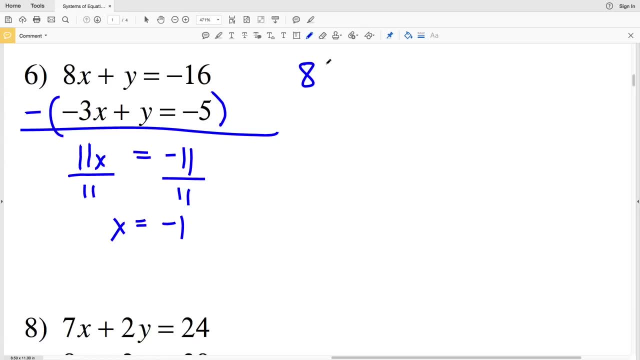 it back in for X in my first equation. so 8 times negative 1, since X is equal to negative 1 plus Y. since we're solving for Y- we, that's our unknown- that's going to be equal to negative 16. so I'll have negative 8 plus Y plus a positive 3, which is negative 16, plus a positive 3, which is negative. 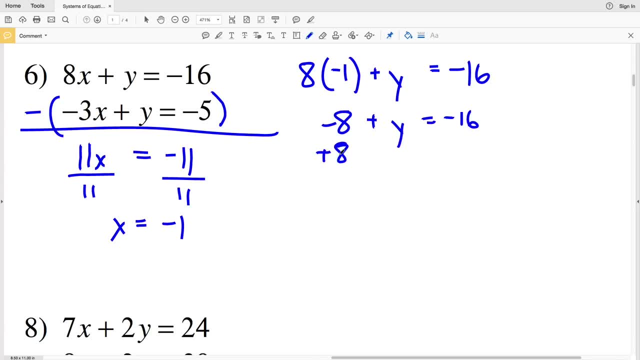 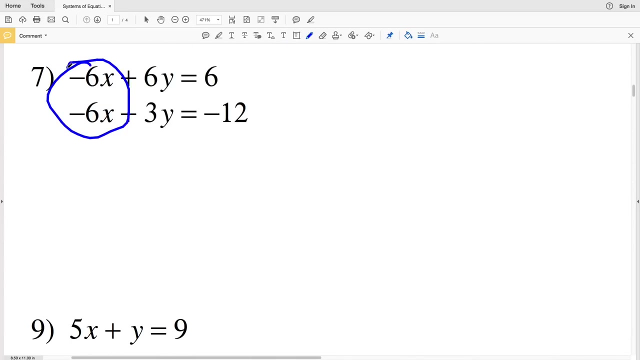 16. so I'll add a positive 8 to both sides in order to isolate my Y variable and I'll get the Y is equal to a negative 8, since negative 16 plus a positive 8 is negative 8. so my solution and number 6 is negative 1, negative 8, a number 7, negative 6 X and negative 6 X, I'll be able to. 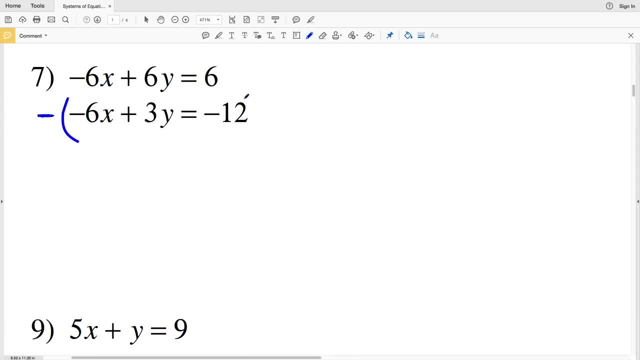 cancel those out by subtracting that second equation from the first. so negative 6x minus a negative 6x is a 0x, which we know is 0. 6y minus 3y is 3y and that's equal to 6 minus a negative 12. 6 plus 12, which is 18. I'll divide both the sides by 3 to get that Y is e with. 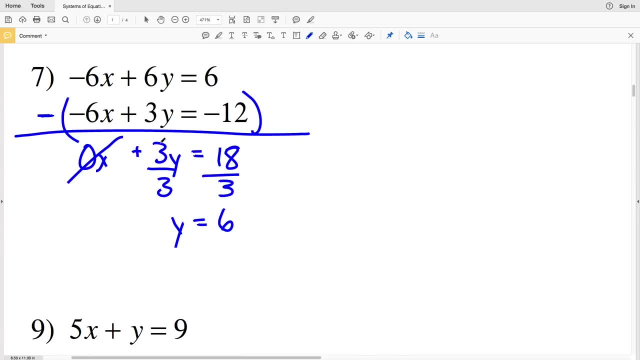 a 6. now that I know what Y is, I'll take Y and plug that in. let's go ahead and use the first equation. so I'm going to subtract my unknown plus 6 times 6, since Y is 6 equals 6, so negative 6x plus 36 equals. 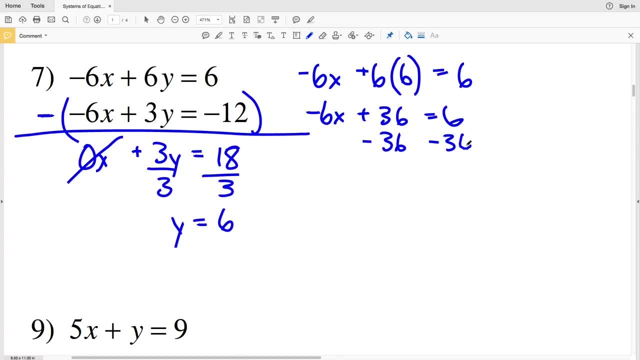 6. if I subtract 36 from both sides, I'll get that negative 6x equals 6 minus 36, which is negative 30. so my next step will be to divide by a negative 6 to get that X is equal to a positive 5, since 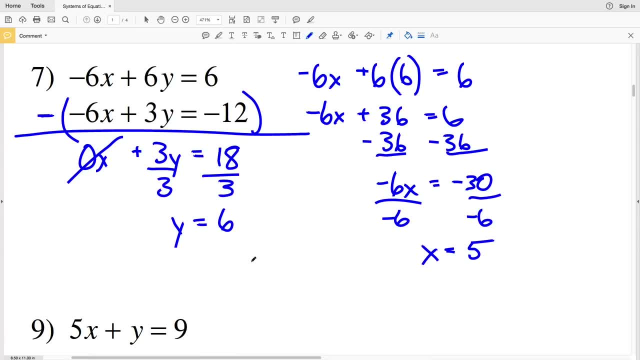 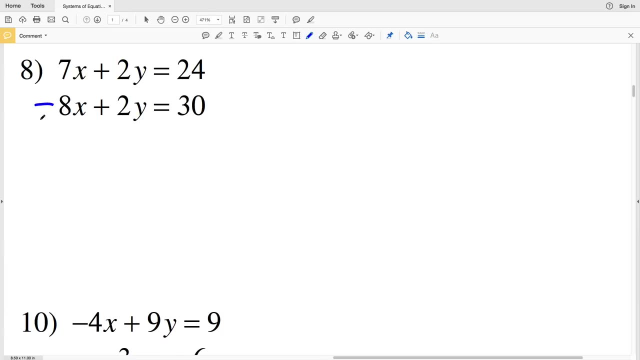 negative 30 divided by negative 6 is 5. so my solution and number 7 is 5 for X and 6 for Y. lastly, in this video I'll go over number 8 and number 8. I'm going to be able to cancel out my 2y by subtracting the equations 7x minus 8x is: 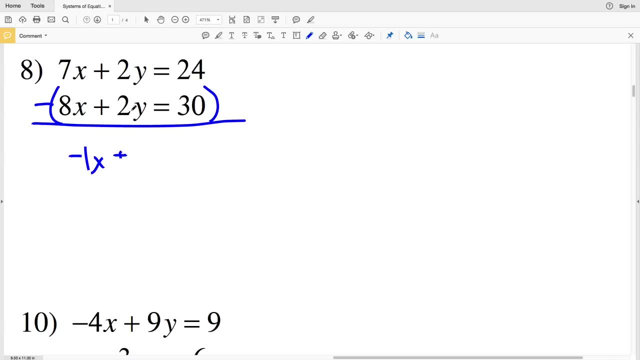 negative 1x. 2y minus 2y is zero y, and 24 minus 30 is negative 6. so minus X is equal to negative 7. so negative 1x is minus 8x or negative 6 is negative 7, and I multiply those by minus x, that's equal to a negative 7x and minus 8 is equal to 6.. 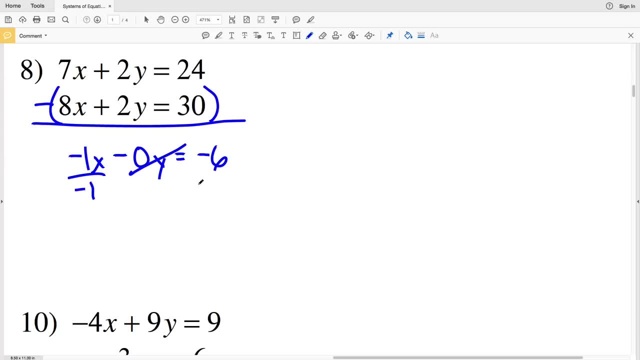 is equal to negative 6. so when I divide both sides by negative 1 I'll get that X is equal to a positive 6. so I'll take that positive 6 value and plug it in for X in my first equation. so 7 times. 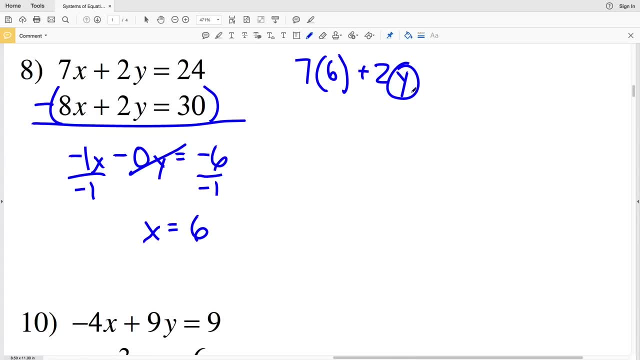 positive: 6 plus 2 times Y- Y's are unknown- is equal to 24. 7 times 6 is 42. so 42 plus 2y equals 24. when I subtract 42 from both sides, I'll get that 2y is equal to a negative 18 and dividing by a positive, 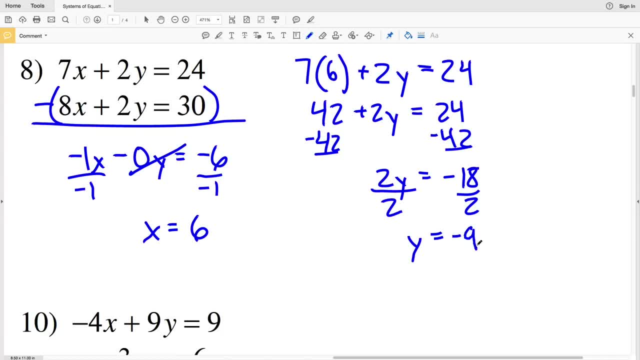 2, I'll get that Y is equal to negative 9 and number 8, X is equal to 6 and Y is equal to negative 9. that's my final solution in this video. join me in the next video, where I'll continue on completing numbers 9 through 16. if you have any questions, leave them in the comment section. 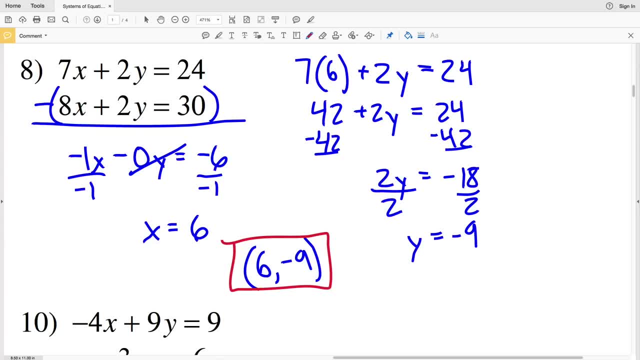 in the comments below and, if you haven't done so already, like, subscribe and share.